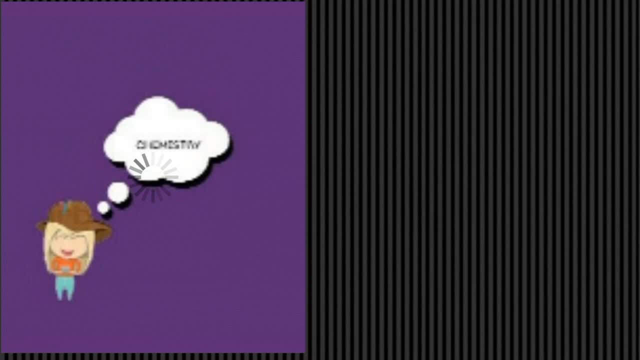 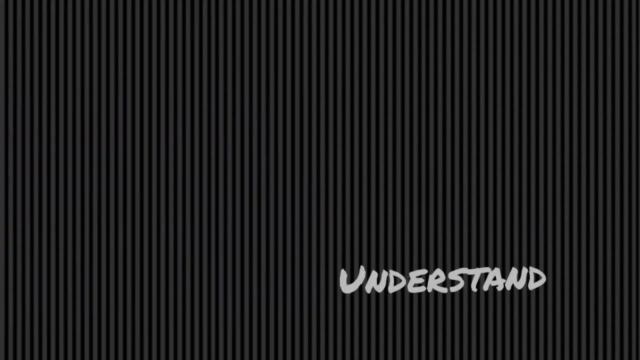 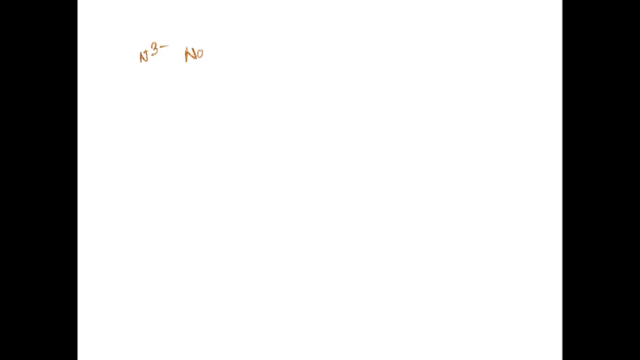 So in our very first question we have comparison of sizes of N3-, sodium+, F-, O2- and Mg2+ And, as I have told you, we will discuss about group 1-2 element. but our first question is a very basic radius question. 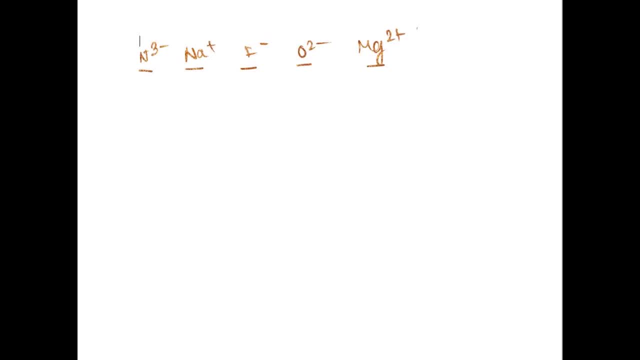 That's why I have given you a very basic radius question. So let's get started. So I have kept that question. So here, whenever we have such type of question, we know that anion having more chard will have the highest size. 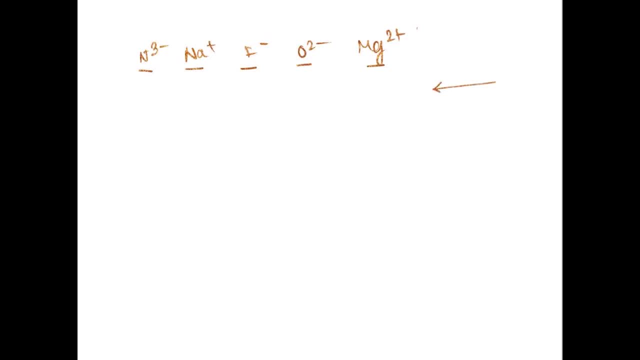 And then we have to consider the PAD. trend also means from right to left the size of the atom increases. So that thing also Okay. so our very first question is increasing order of ionic size. So we have here N3-, sodium+, O2-. 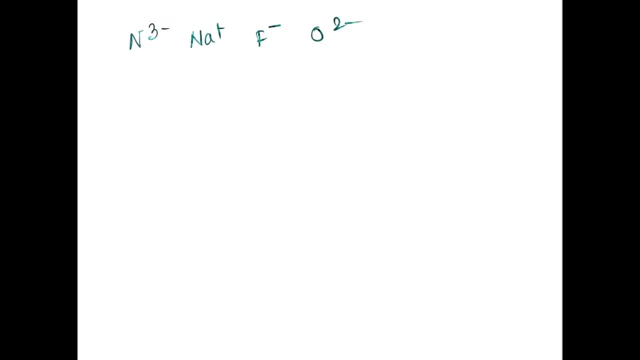 F-, O2- and Mg2+. Now you look, whenever we are going for ionic size. so ionic size means size of that ion, And size of that ions depends on charges and on the atomic number also. Now, mutually we will take actually Z and E ratio. 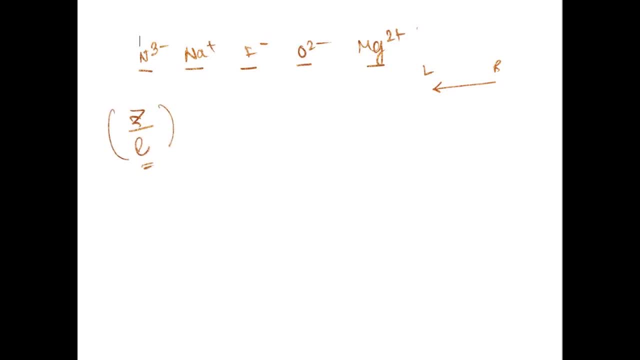 So in Z and E ratio here total number of that electron we can see. for nitrogen total number of electron will be 10 for sodium plus 10, for fluoride minus 10, for oxide 10 and H2O2 plus 10.. 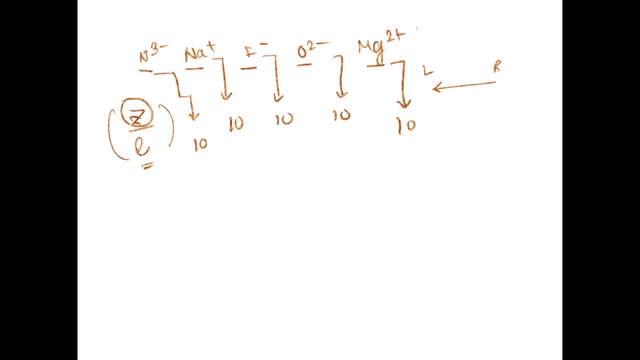 So here Z by E ratio will completely depends upon N, completely depends upon Z. So higher the Z means higher the negative charge, higher will be the. that radius means size. So here size 10 will be in the increasing order. So first we will write sodium plus, then there will be magnesium 2 plus, then there will be F-, then O2- and at the end N3- 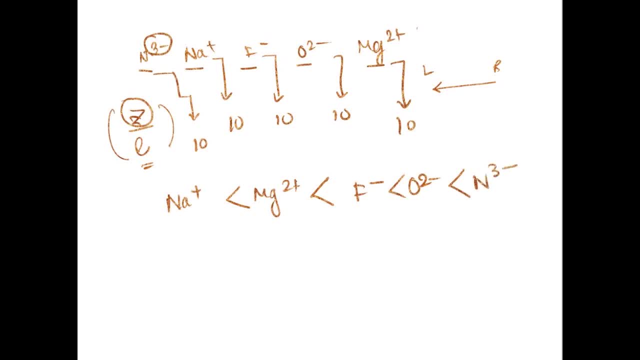 So for the basic concept I have kept this way. So in the next there is decreasing thermal stability, decreasing thermal stability of group 2, metal ion sulfate, And Here We have barium sulfate- BeSO4,, magnesium sulfate- NGSO4,, calcium sulfate- CaSO4, and strontium sulfate- SrSO4. 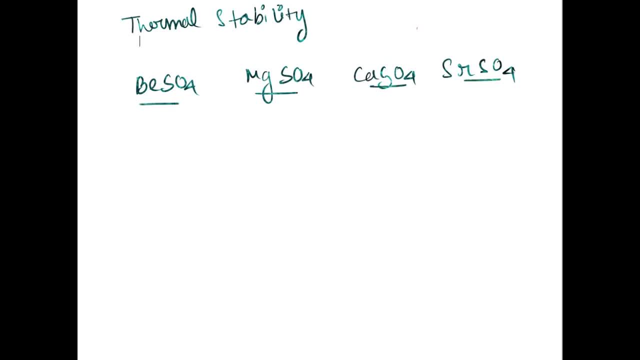 Now the thing is, when we are considering this, we will take here: the cation is beryllium 2 plus and anion is SO4 2 minus. Here magnesium 2 plus and SO4 2 minus. Calcium 2 plus and SO4 2 minus. 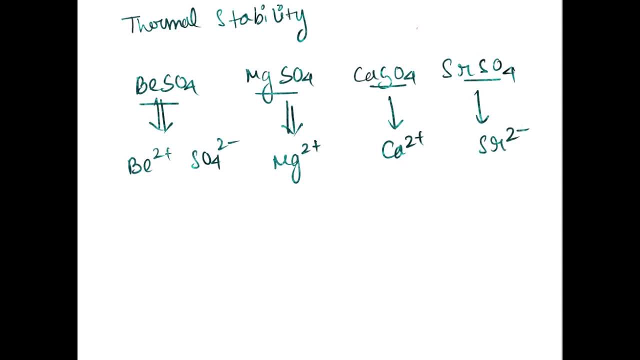 Calcium 2 plus and SO4 2 minus, Calcium 2 plus and SO4 2 minus minus, and here strontium 2 plus and SO4 2 minus. so for thermal stability, as we know, sulphate ion is a large anion. so for this large anion, the thing will: 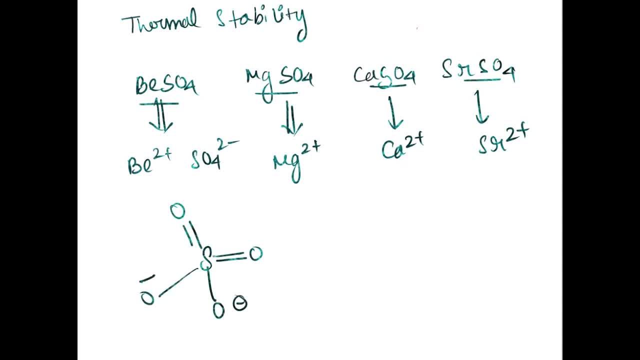 be like SO4 2 minus, like this. so if it binds with larger cation, so that binding will be more prominent and that's why, with increasing the size of the cation, the interaction between anion cation will be good, means the bonding stability will be better. that's why the stability trend will be like: 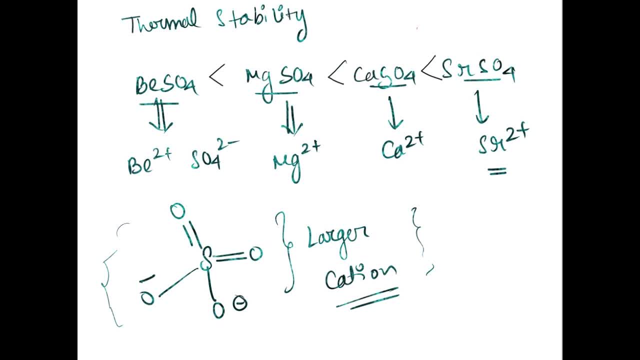 barium sulphate, magnesium sulphate, calcium sulphate, strontium sulphate. So this one is the increasing stability, as in the question, this is asked to write decreasing stability. so our answer will be strontium sulphate first, then calcium sulphate, then magnesium sulphate tomorrow. our answer will be: 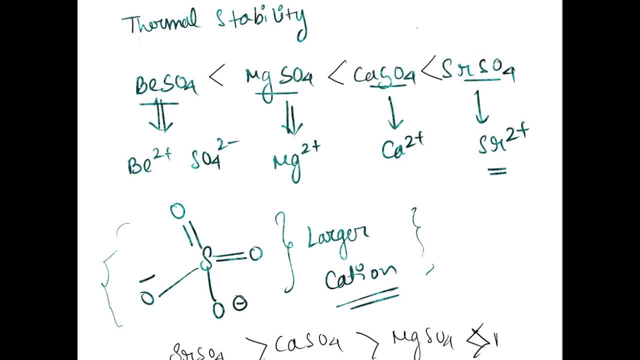 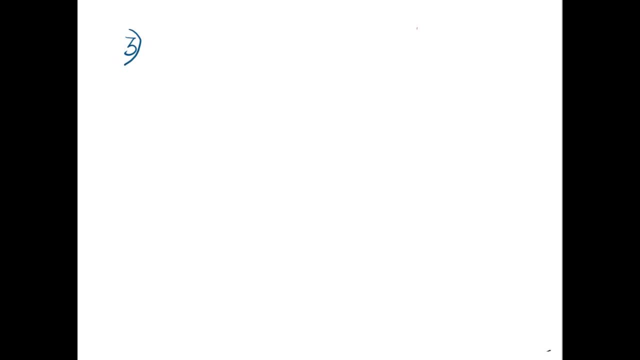 sulfate and at the end barium sulfate, moving towards the third question. third question was arrange them in increasing order of their metallic character. so our elements are boron, aluminium, magnesium, potassium. now to arrange them in increasing metallic character, we have to know what does that metallic character? 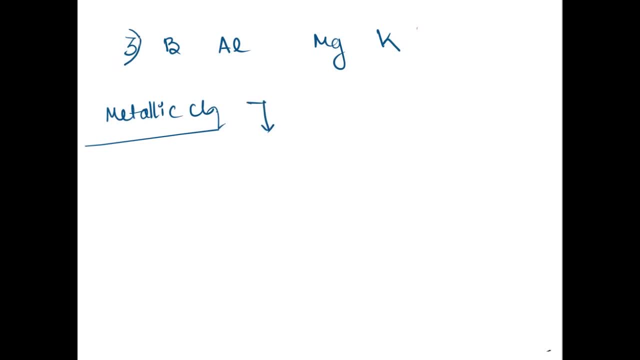 metallic character means any element that having tendency to lose its electron and to form positive charge, will be called metal. that means which elements have the higher tendency to form positive charge, more metallic in nature. so, as here you can see, here the elements are boron aluminium, magnesium. 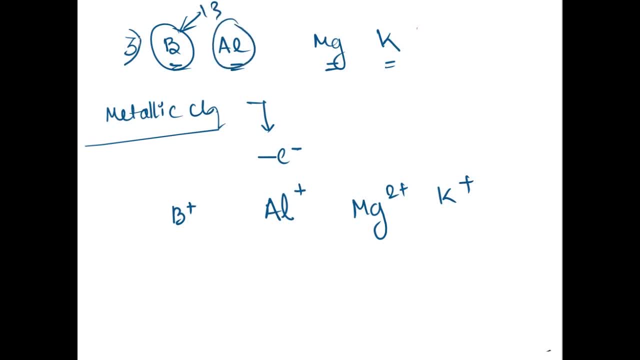 potassium, boron is from group 13, aluminium is from group 14. so our group one two element is potassium, group one, magnesium group two. so here, the more we go from right side to left side, size of the atom increases, increases and more tendency to give electron increases. that's why metallic 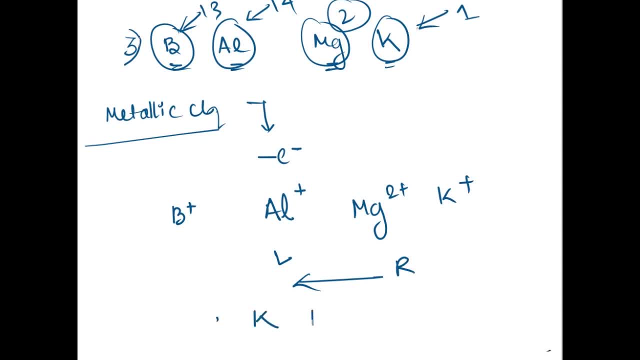 character will be higher for potassium and magnesium, and magnesium metallic character will be higher than boron, and boron having more than aluminium. that another thing which act means in between, in between the two are boron and aluminum. boron is aluminum is in the third period, whereas boron is in the second period. 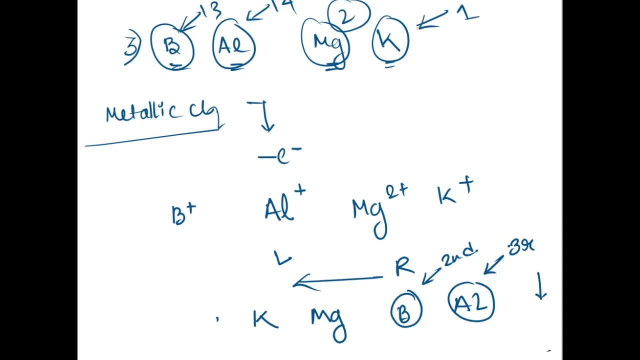 now, if we go up to down, then also metallic character increases. that's why here most metallic will be nature, potassium, then magnesium, then aluminium and at the end boron. so that will be the trend in the increasing order of metallic character. now for the fourth question. there is: 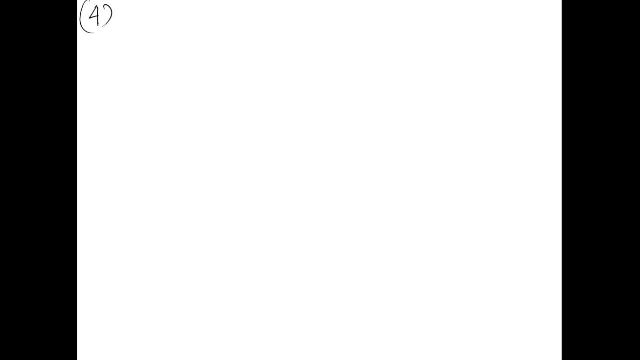 increasing order of carbonate. stability of group two elements. so we have barium carbonate, we have magnesium carbonate, we have calcium carbonate and strontium carbon. now again from for carbonate. so if we see carbonate as an anion, so carbonate is a large anion. so here, 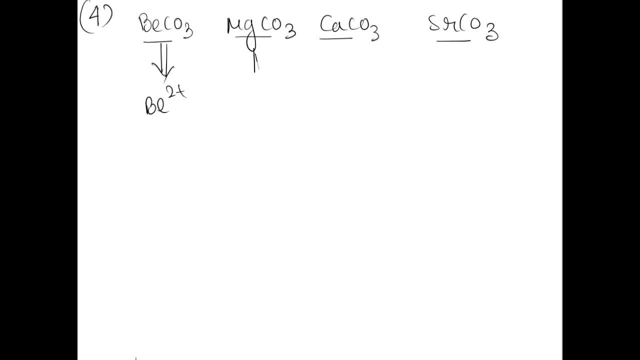 the cations are changed. so here, beryllium 2 plus, magnesium 2 plus, calcium 2 plus and strontium 2 plus we have. so here in all that cation, when cation is attaching with larger anion, so that interaction will be better. that's why carbon stability will be. 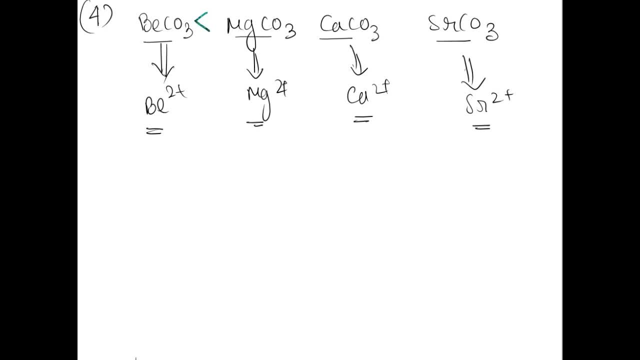 in that, in this trend, when we will go from beryllium towards strontium, the carbonate stability will increase. so this will be the trend. now i am moving towards the fifth question. so our question is: basic character of hydrides. so what we have? we have group one, hydrohydroxide. 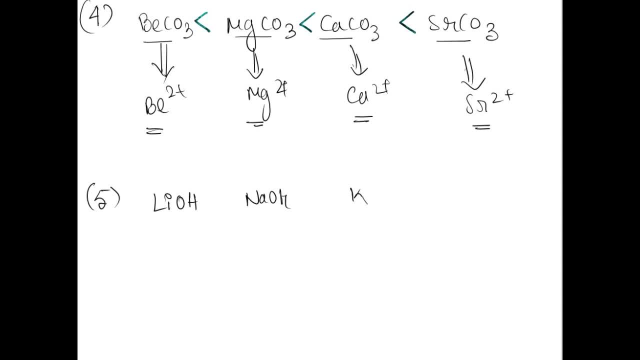 lithium hydroxide, sodium hydroxide, potassium hydroxide and rubidium hydroxides. so if we want to see the basic character, so basic character means the tendency of that particular hydroxide to donate hydroxide ion, ru minus an, so more the tendency to donate hydroxide ion, more will be the. 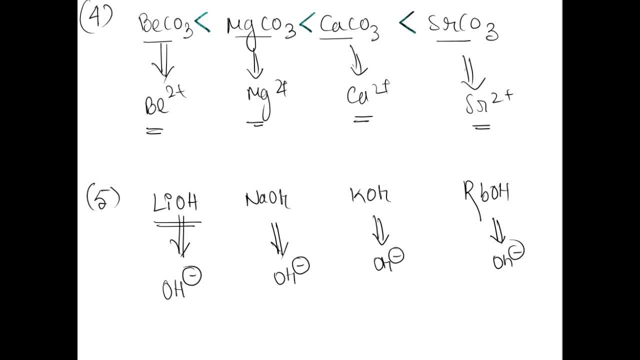 basicity. now, if we go up to down, we know the size of the element increases. so because of increase of size, the element have more tendency to donate its electron and have more tendency to form lithium plus, sodium plus, potassium plus and rubidium plus. that's why, with more tendency of 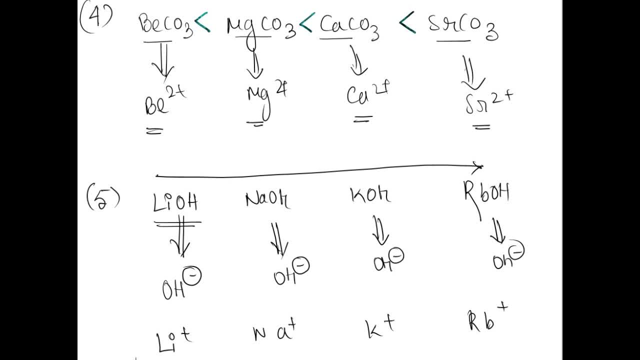 forming for cation, there is a more tendency of forming hydroxide ion also, so that's why basicity, or basic strength, will be in the order from left to right. the increasing basic strength will be lithium hydroxide, sodium hydroxide, potassium hydroxide and rubidium hydroxide. 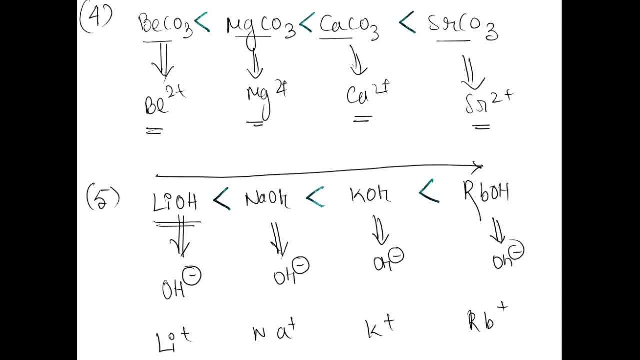 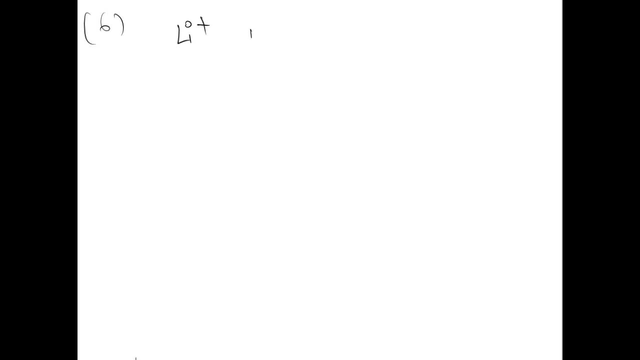 now moving towards our sixth question. okay, our sixth question is radii of hydrated cation of group B one: lithium, sodium, potassium and rubidium. now, whenever we're considering only the cation size, the cation size order will be in this order, but they want the strength of hydrated ion hydrated. 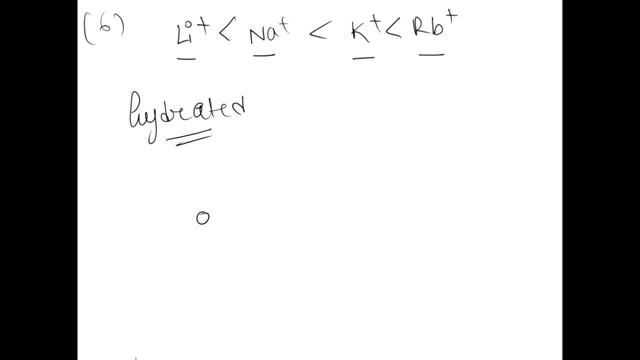 cation size, so the smaller will be the cation, more will be. this one means water molecule will surround it more, so smaller. one is lithium positive, so more water molecule will be there around lithium positive, so hydrated ions size will be more. for smaller cation, the larger the cation, less water molecule. 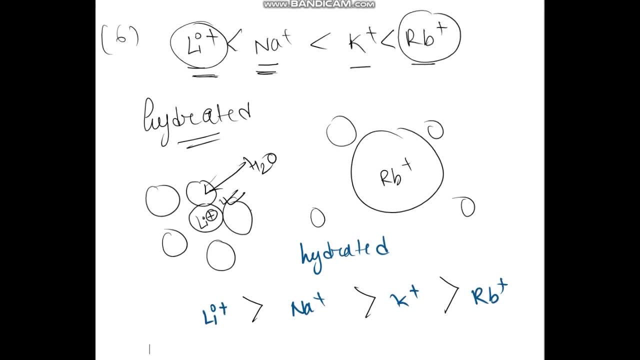 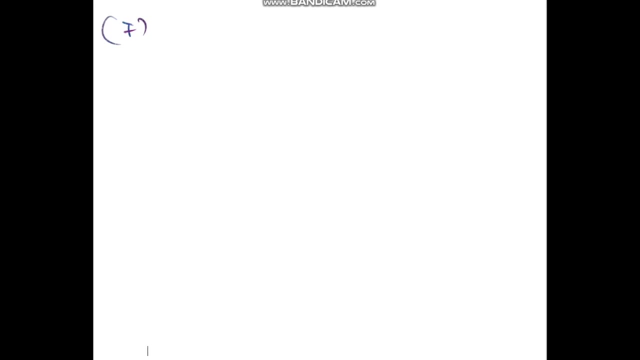 will be there. so because of the smaller size, more water molecule will be there. so hydrated cation trend will be highest for lithium positive and lowest for rubidium positive. now moving towards seventh question. so our seventh question is here. it is asked to arrange them in the electronegativity. 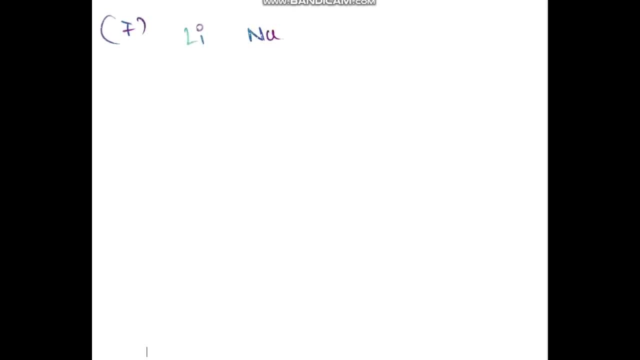 chain. so this one is the most easiest. question means if we are trying to arrange the electronegativity chain. as we know, if we go from up to down in a periodic table to electronegativity decreases. so lithium in the uppermost position, ccm in the lowermost electronegativity. 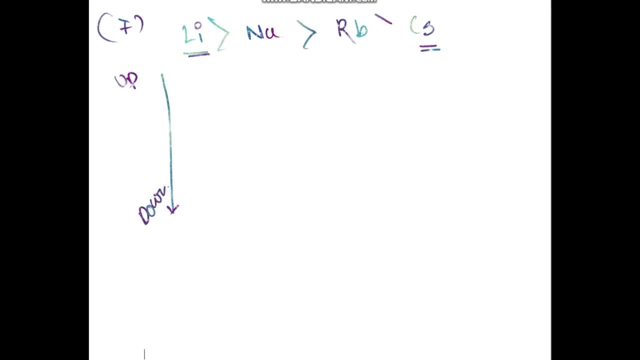 trains will be lower from I, from up to down, from lithium to ccm. electronegativity emprend will decrease. now moving towards question number eight. now in question number one is Question number 8, it is asked to arrange them in the solubility order. 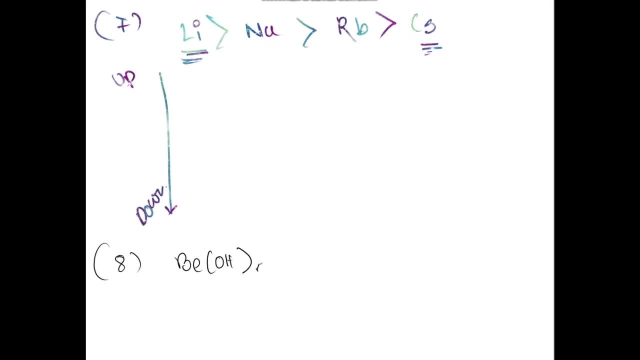 The hydroxide of group 2 ion in solubility order: Bainium hydroxide, calcium hydroxide and strontium hydroxide. So if we are taking this and we are seeing the solubility order, So always remember more- it can give cation and anion in water or in any solvent. 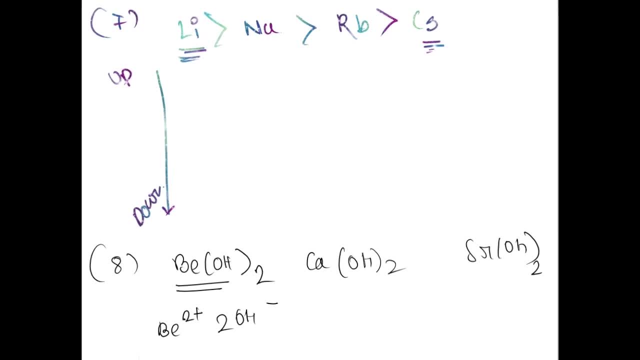 The more solubility will it face. So, as we know, if we go from up to down, electropositivity character increases. So that's why more giving tendency of more cation and anion will increases from bainium to strontium. 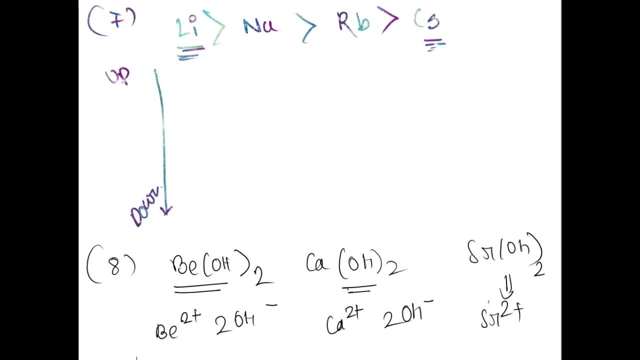 So that's why solubility trend will be here like this way: Bainium hydroxide, calcium hydroxide, then strontium hydroxide, Then our 9th way, arrange the following in there: Increasing order of ionic character. 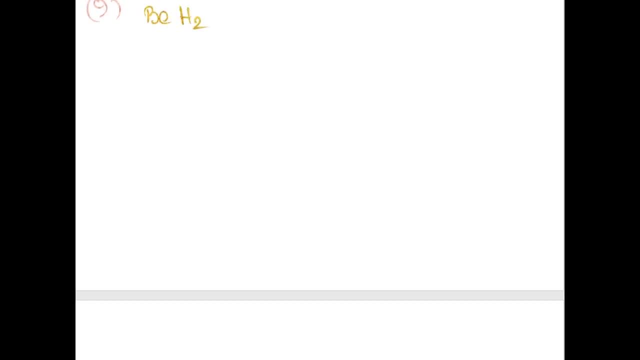 We have some hydrides of group 2. Methylene, so bainium hydride, magnesium hydride and calcium hydride. So, as you can see, hydride is of small anion, So it will go more with the large means, the larger the cation.